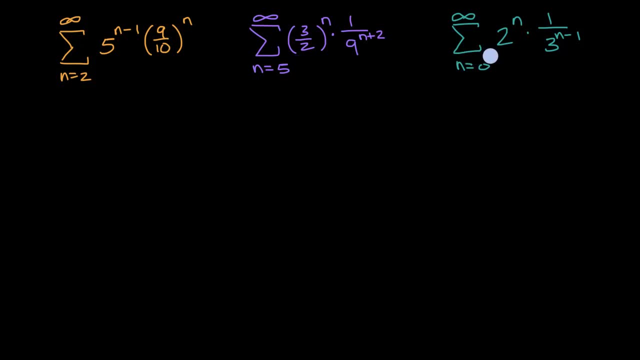 So here we have three different series, and what I would like you to do is pause this video and think about whether each of them converges or diverges. All right, now, let's work on this together. So, just as a refresher, converge means 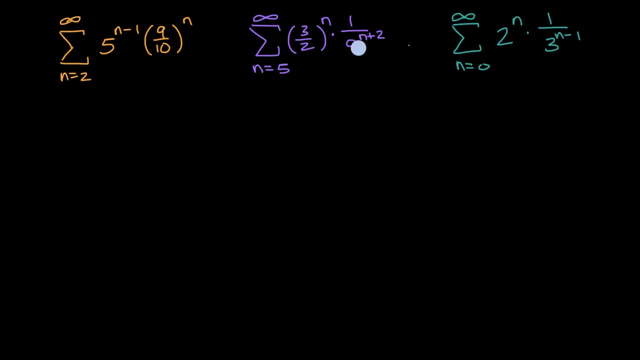 that, even though you're summing up an infinite number of terms, in all of these cases, if they converge, that means you actually get a finite value for that infinite sum or that infinite number of terms being summed up, which I always find somewhat amazing. 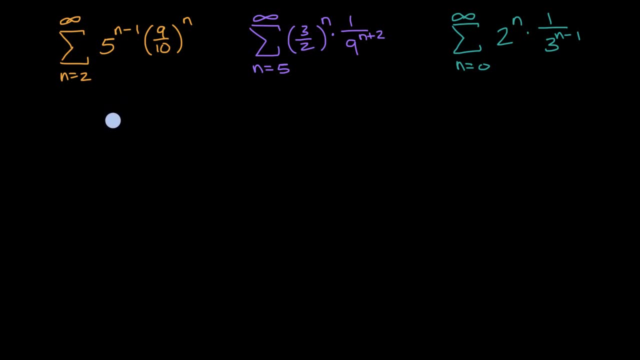 and diverging means that you're not going to get an actual finite value for the sum of all of the infinite terms. So how do we think about that? Well, we already know something about geometric series, and these look kinda like geometric series. 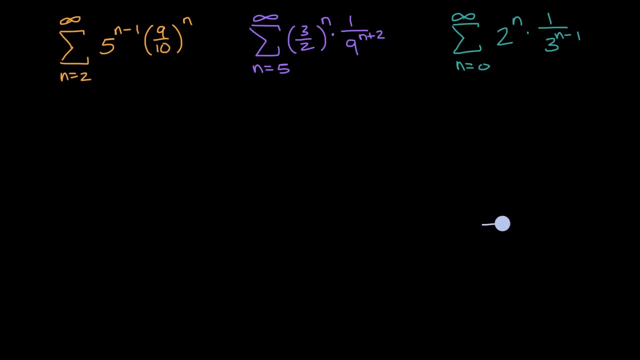 so let's just remind ourselves what we already know. We know that a geometric series, the standard way of writing it is we're starting, n equals. typically you'll often see n is equal to zero, but let's say we're starting at some constant. 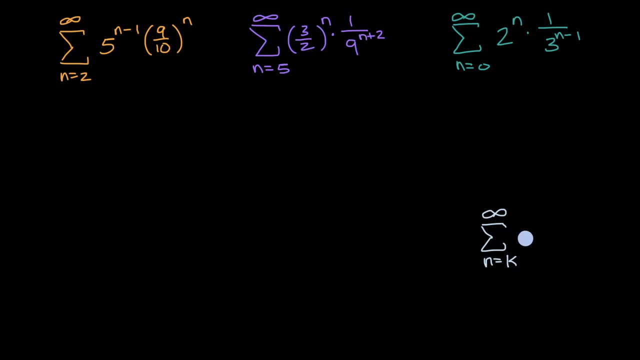 and then you're going to have- you're going to go to infinity- of a times r to the n, where r is our common ratio. We've talked about that in depth in other videos. We know this is the standard way to write a geometric series. 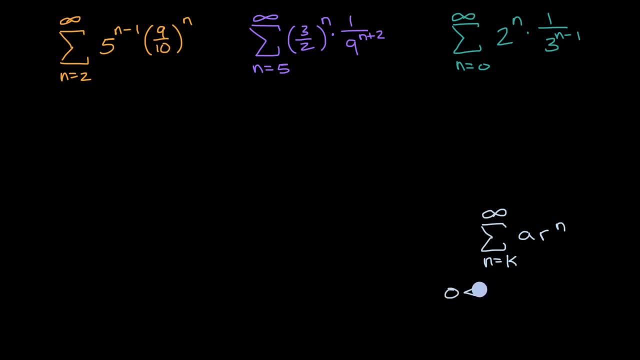 We know that if the absolute value of r is between zero, is between zero and one, then this thing is going to converge, converge, and if it doesn't, I'll just write it, else it will diverge. So maybe a good path would be. 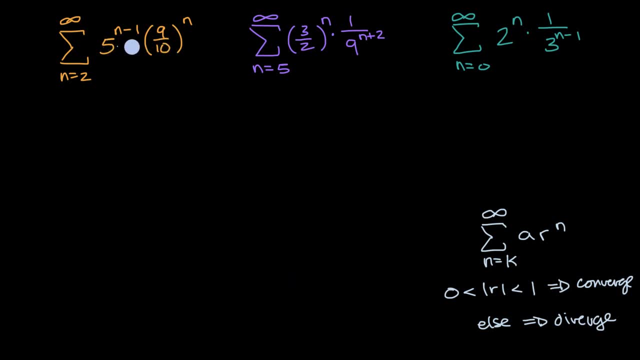 hey, can we rewrite these expressions that we're trying to take, that are defining each of our terms as we increment n? If we can rewrite it in this form, then we can identify the common ratio and think about whether it converges or diverges. 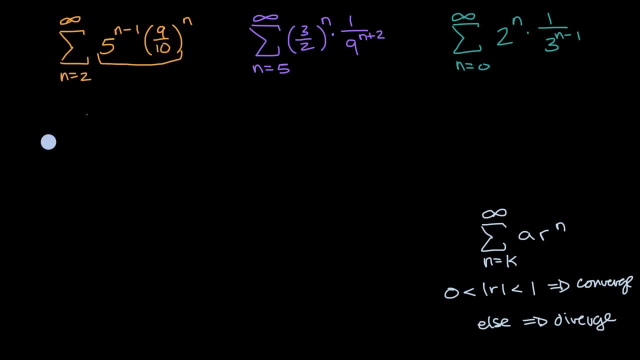 So I'm going to focus on this part right over here and see if I can rewrite that. So let's see, can I rewrite five to the n minus one? I can rewrite that as five to the n times five to the negative one. 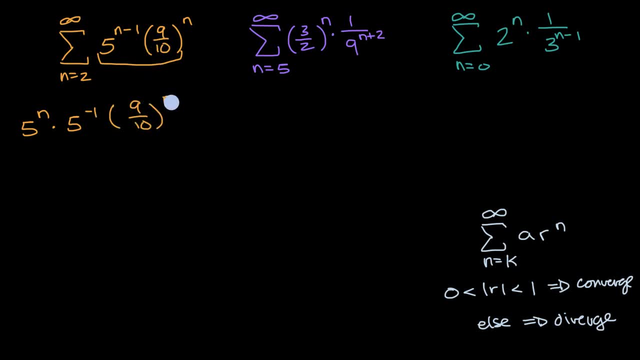 and then that's going to be times nine-tenths to the n. And let's see, this is going to be equal to it's going to be. I could just write this as this part right over here. I'll write as one-fifth. 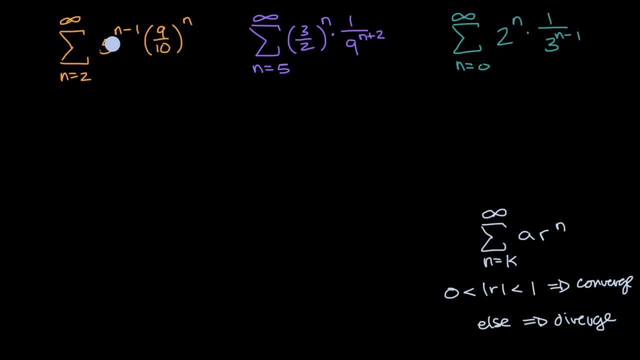 hey, can we rewrite these expressions that we're trying to take, that are defining each of our terms as we increment n? If we can rewrite it in this form, then we can identify the common ratio and think about whether it converges or diverges. 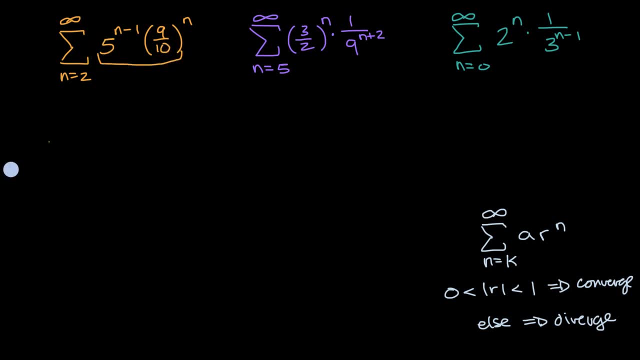 So I'm going to focus on this part right over here and see if I can rewrite that. So let's see, can I rewrite? let's see five to the n minus one. I can rewrite that as five to the n minus one. 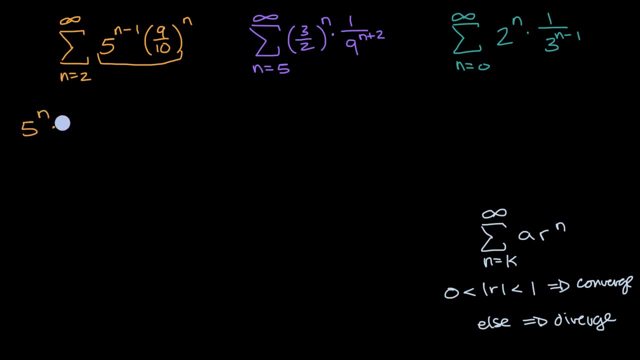 Let's see: five to the n minus one. I can rewrite that as five to the n minus one, five to the n times five to the negative one, and then that's going to be times nine, tenths to the n, And let's see this is going to be equal to. 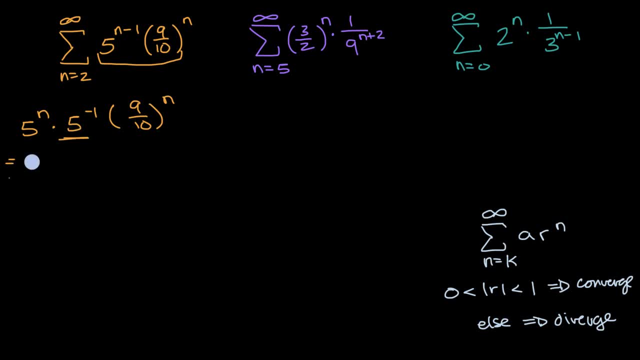 it's going to be. I could just write this as this part right over here. I'll write as one fifth, that's the same thing as five to the negative one times, and then five to the n and nine tenths to the n. 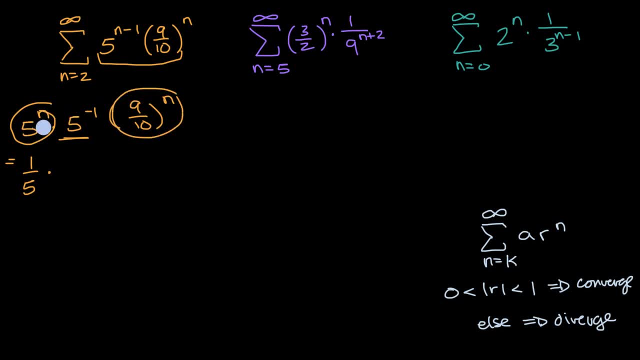 well, I have the same exponent, so I can rewrite that as: and we're multiplying all this stuff. I'm just switching the order. this is the same thing as five times nine tenths to the nth power, and so this is going to be equal to one fifth times. 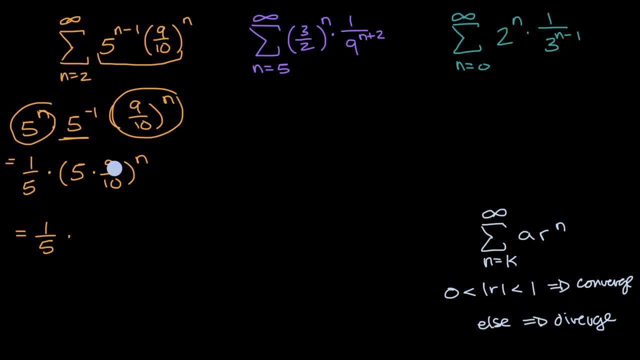 well, five times nine is 45,. divided by 10, is going to be 4.5, so times 4.5 to the nth power, So that original series I could rewrite as just for good measure I'm starting at n- equals two. 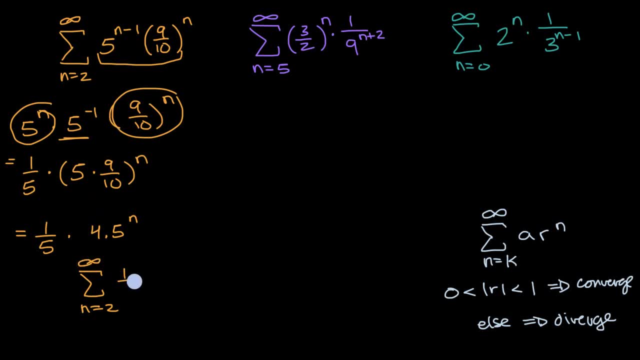 I'm going to infinity, and this could be rewritten as one fifth times 4.5 to the n. So what's our common ratio? what's our R here? Well, you can see very clearly: it is 4.5.. The absolute value of 4.5 is clearly not between zero and one. 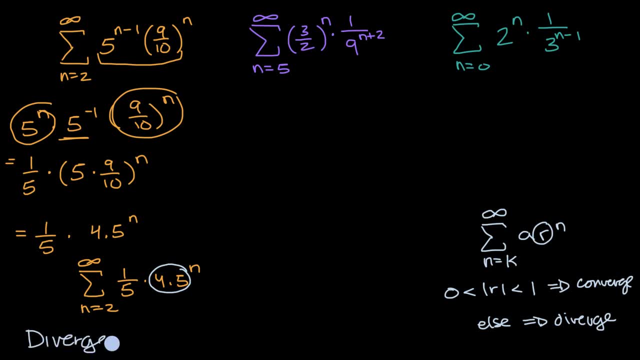 so this is a situation where we are going to diverge Now. if you found that inspiring and if you weren't able to do it the first time, I asked you to pause the video, try to pause the video again, the video again and try to work these out now. 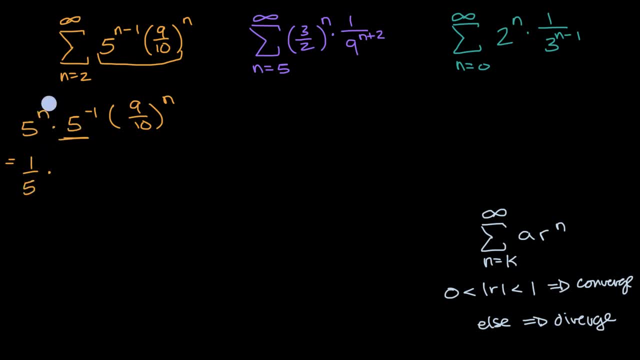 that's the same thing as five to the negative one times and then five to the n and nine-tenths to the n. well, I have the same exponent, so I can rewrite that as before, multiplying all this stuff. I'm just switching the order. 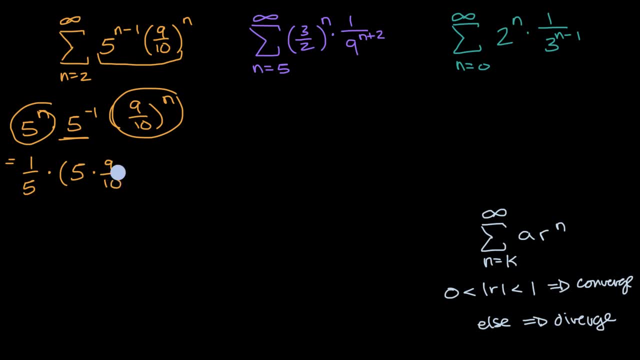 this is the same thing as five times nine-tenths to the nth power, and so this is going to be equal to one-fifth times. well, five times nine is 45,. divided by 10 is going to be 4.5,. 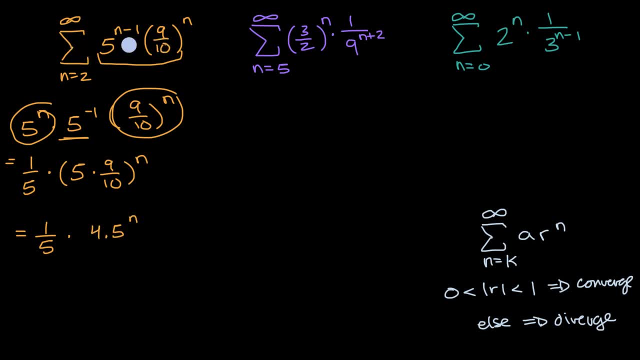 so times 4.5 to the nth power, So that original series I could rewrite as just for good measure, I'm starting at: n equals two, I'm going to infinity, and this can be rewritten as one-fifth times 4.5 to the n. 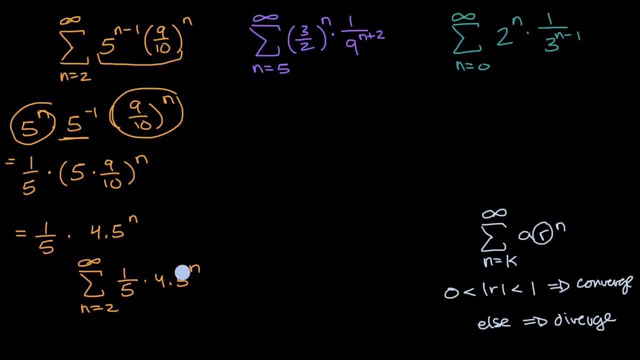 So what's our common ratio? what's our r here? Well, you can see very clearly, it is 4.5.. The absolute value of 4.5 is clearly not between zero and one. so this is a situation where we are going to diverge. 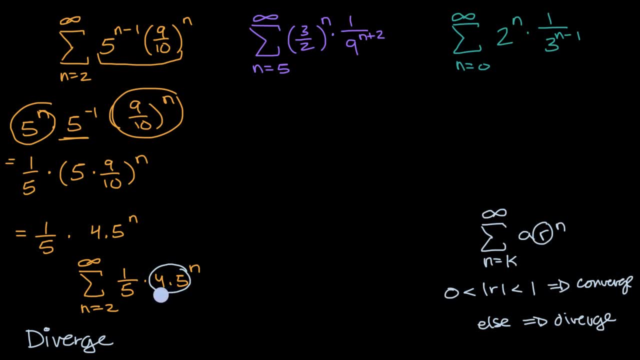 Now, if you found that inspiring, and if you weren't able to do it the first time, I asked you to pause the video- try to pause the video again and try to work these out now. now that you've seen an example, All right, let's jump into it. 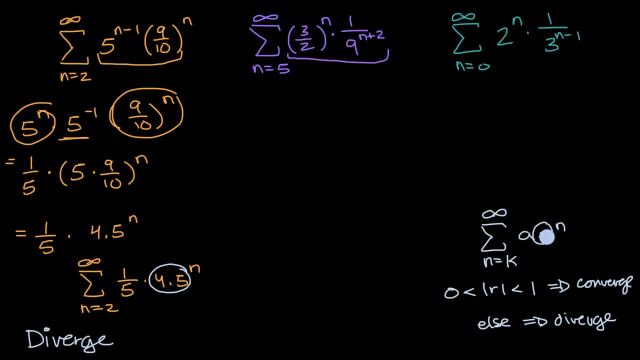 So I'm just going to try to algebraically manipulate this part to get it into this form. so let's do that, So I could rewrite this. let's see if I could get some things just to the nth power, so I could rewrite it. 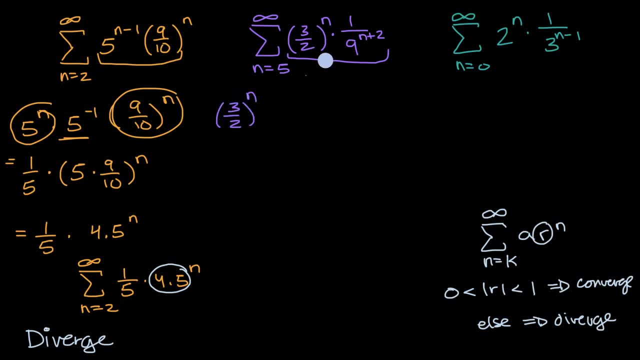 as three-halves to the nth power, and I could write this part right over here as times one over nine to the nth. times nine squared, this is going to be equal to three-halves to the n, and let's see I could factor out. 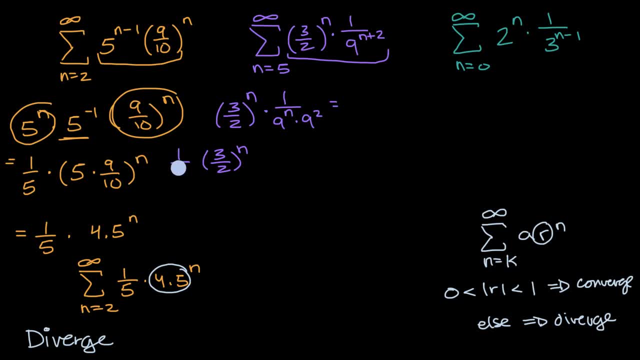 or bring out the one over nine squared. so let me do that, so I'll write that as one over 81, I'll write it out there. so that's this part right over there. 181 times three-halves to the n, times one over nine to the n. 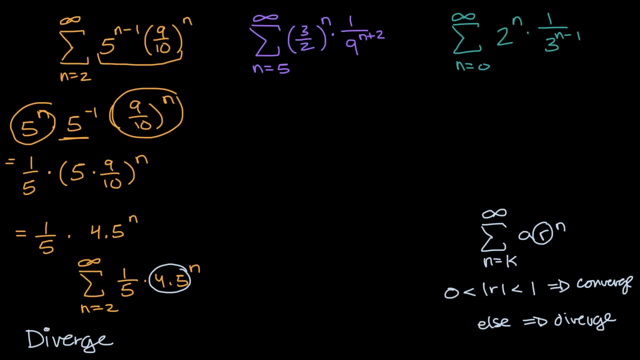 now that you've seen an example, All right, let's jump into it. So I'm just going to try to algebraically manipulate this part to get it into this form. so let's do that. So I could rewrite this. let's see. 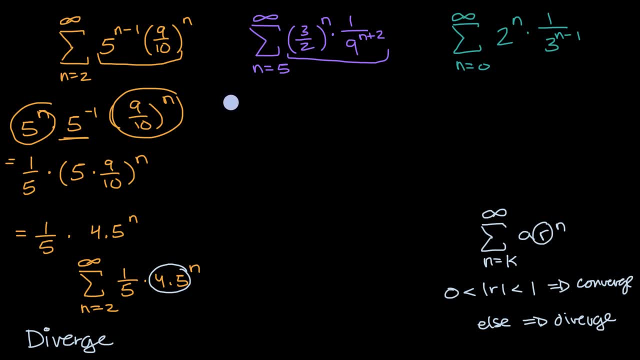 if I could get some things just to the nth power, so I could rewrite it as three halves to the nth power and I could write this part right over here as times one over nine to the nth. times nine squared, This is going to be equal to three halves to the n. 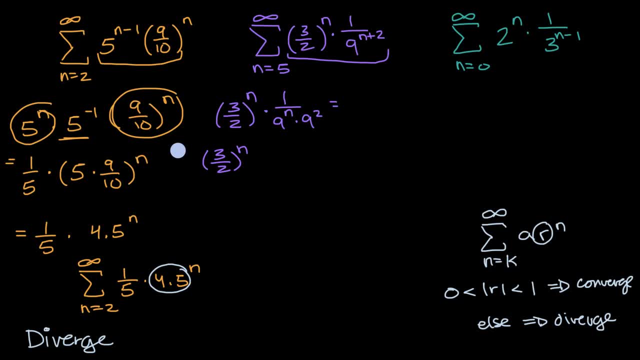 And let's see, I could factor out or bring out the one over nine squared. so let me do that. so I'll write that as one over 81.. I'll write it out there. so that's this part right over there. 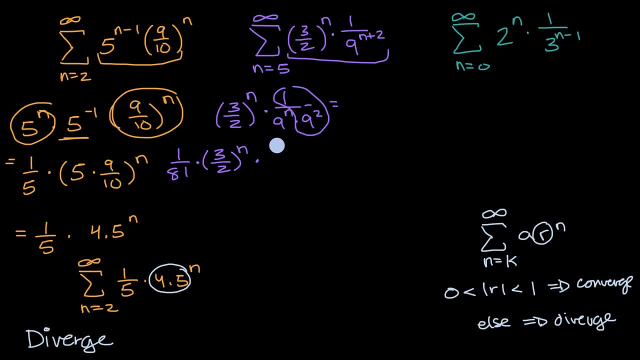 181 times three halves to the n, times one over nine to the n, But one over nine to the n. that is the same thing as one over nine to the n, One over nine. all of that to the nth power, And the reason why I did that is now I have 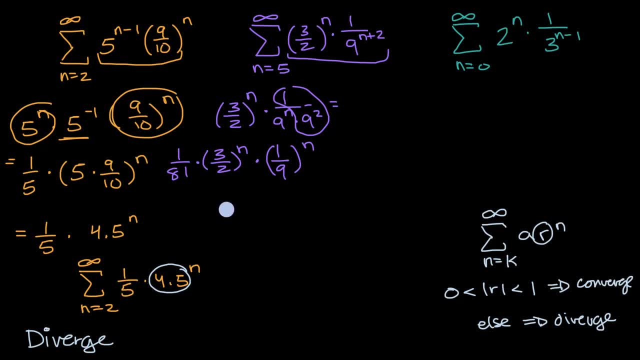 both of these things to the nth power, and I can do just what I did over here before. So this is all going to be equal to one over 81 times three halves times one ninth to the nth power. These are just exponent properties that I am applying right over here. 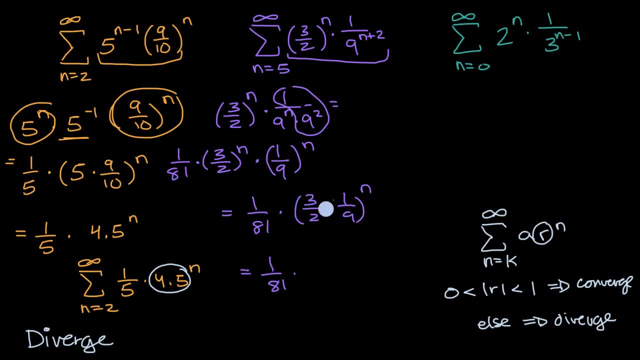 And so this is going to be equal to one over 81 times. let's see three halves times one over 81.. One over 81 times one. ninth is 3 18ths, which is the same thing as one sixth times one. sixth to the nth power. 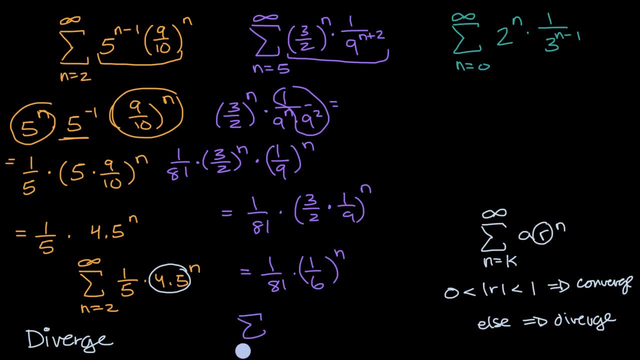 Or if I were to rewrite the original series, it's: the sum from: n equals five to infinity of of now I can rewrite it as one over 81 times one sixth to the nth power. This is our common ratio. one sixth, very clearly. 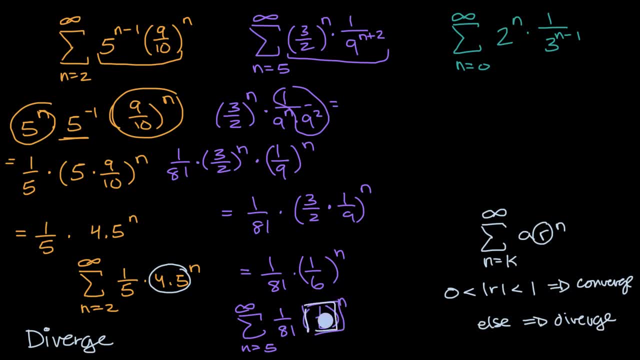 I'll do that in this light blue color, Blue color. one. sixth, That absolute value is clearly between zero and one. So this is a situation where we will converge, converge. Now let's do this last example. I'll do this one a little bit faster. 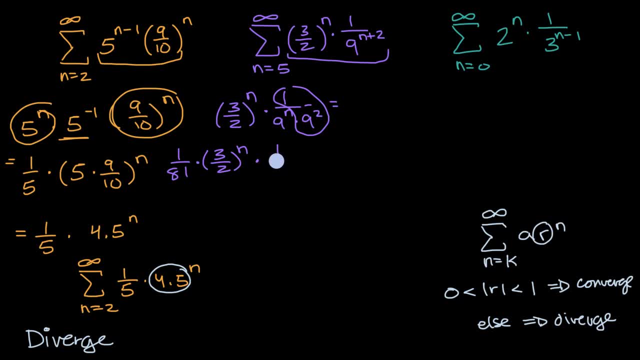 but one over nine to the n. that is the same thing as one over nine. all of that to the nth power, And the reason why I did that is now I have both of these things to the nth power and I can do just what I did over here before. 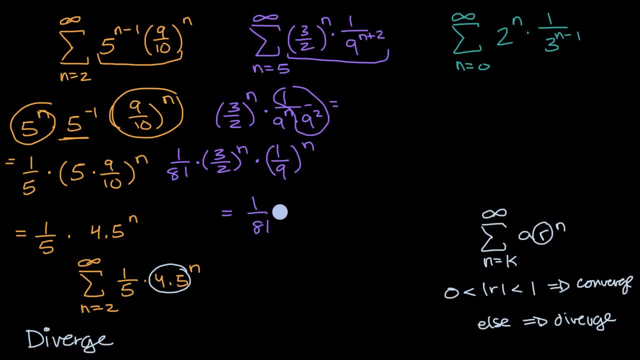 So this is all going to be equal to one over 81 times three-halves times one-ninth to the nth power. These are just exponent properties that I am applying right over here, and so this is going to be equal to one over 81 times, let's see three-halves. 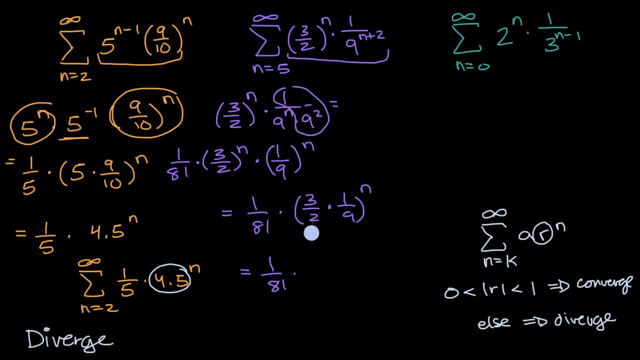 times 1, 9th is 3, 18ths, which is the same thing as 1, 6th times 1, 6th to the nth power. Or, if I were to rewrite the original series, it's: the sum from n equals five to infinity of. 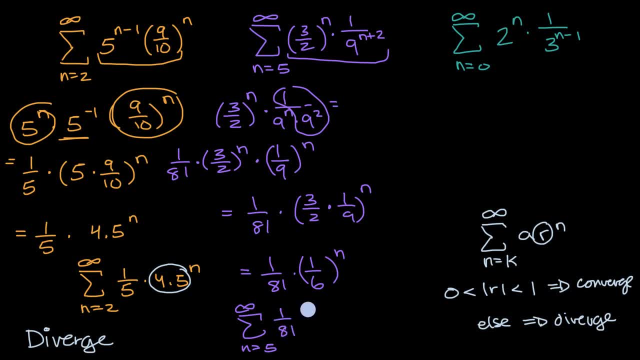 of now I can rewrite it as one over 81, times 1: 6th to the nth power. This is our common ratio: 1: 6th. very clearly, I'll do that in this light blue color: 1, 6th. 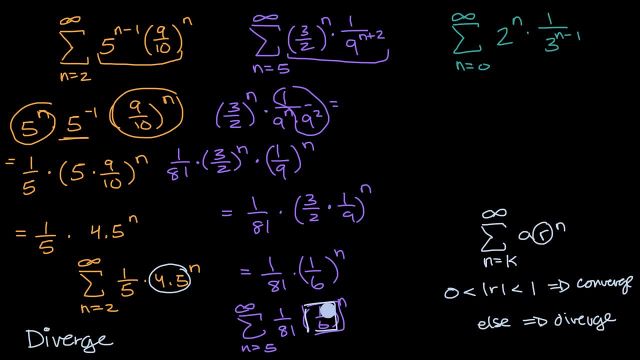 That absolute value is clearly between zero and one. So this is a situation where we will converge, converge. Now let's do this last example. I'll do this one a little bit faster. So let's see I could, if I'm just trying. 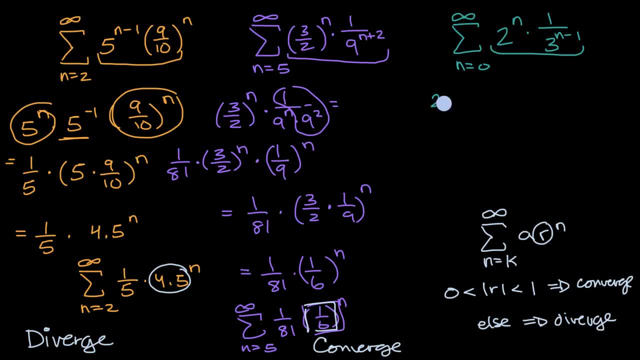 to algebraically manipulate that part there. that's going to be the same thing as two to the nth power times one over three to the n times three to the negative one. Well, this is going to be the same thing as two to the n. 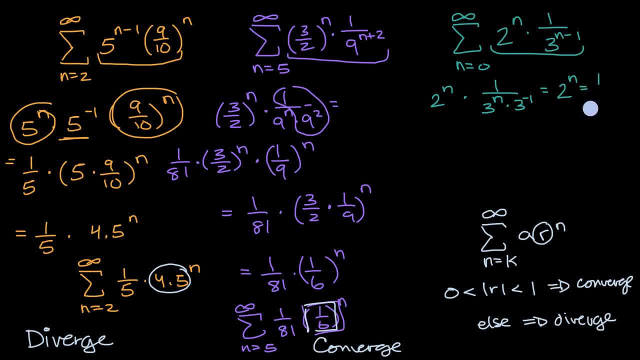 times one over. why did I write equals Times, one over three to the n and one over three to the negative one. That's the same thing as one over 1. 3rd, That's just going to be equal to three. 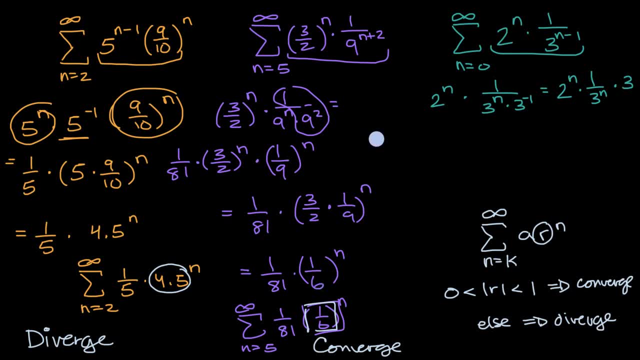 times three. Well, that's going to be equal to: I'll give myself some space, We'll start out here. That's equal to: I'll put the three out front: three times, three times two to the n times and one over three to the n is the same thing. 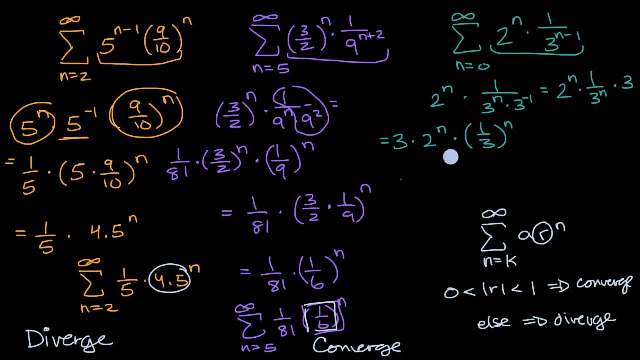 as 1- 3rd to the nth power, And so this is going to be equal to three times two times 1- 3rd, all of that to the nth power, And so that's going to be equal to three times 2 3rds to the nth power. 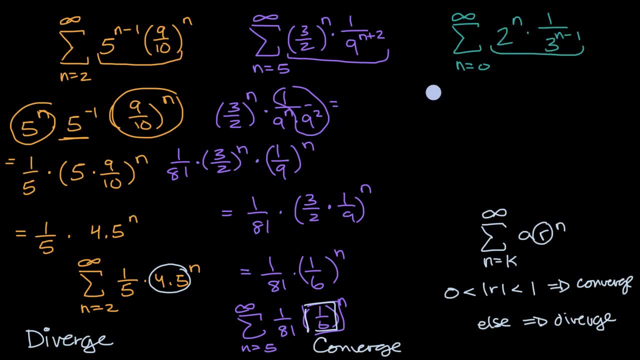 So let's see I could, if I'm just trying to algebraically manipulate that part there, that's going to be the same thing as two to the nth power times one over three to the n times three to the negative one. Well, this is going to be the same thing as two to the n.